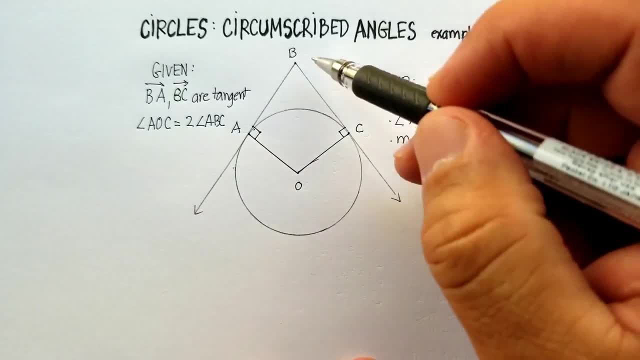 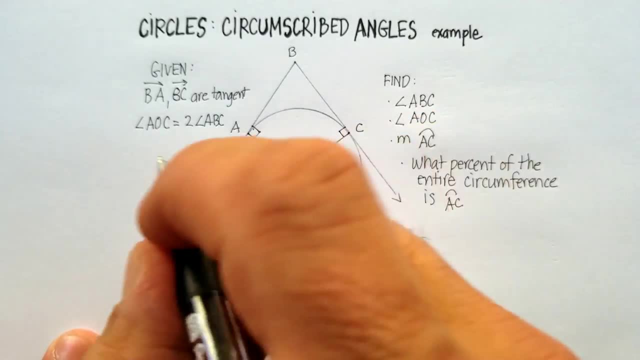 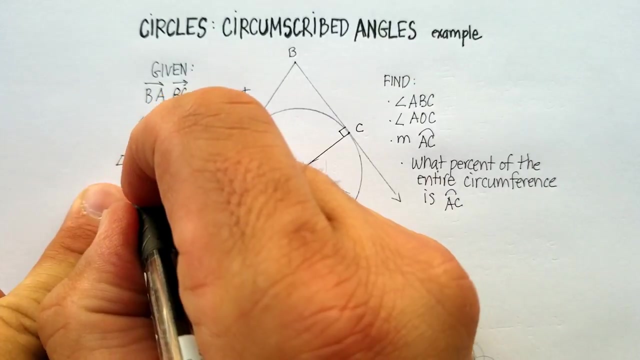 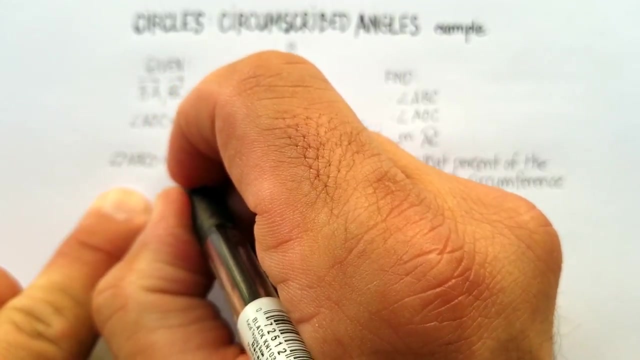 that as soon as I drew the tangent line, I created a four-sided figure, And this four-sided figure is called a kite or quadrilateral, And remember that that's how you draw the symbol for quadrilateral. And we know that ABCO is a kite. What do we know about kites? We know that. 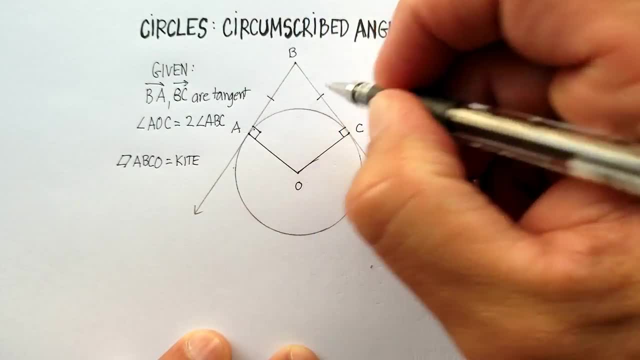 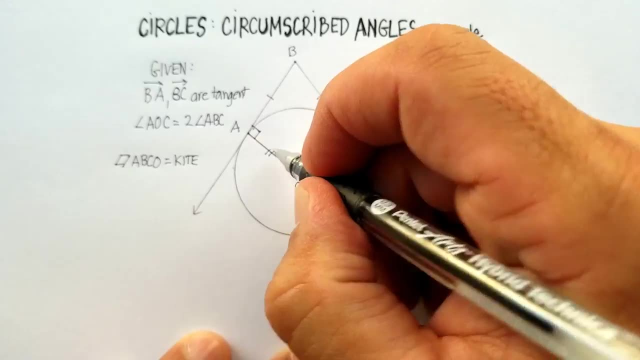 there are two consecutive sides that are congruent. So this side is congruent to this side and then this following side is congruent to this side. Does that help us A little bit? it might. We also know that any quadrilateral 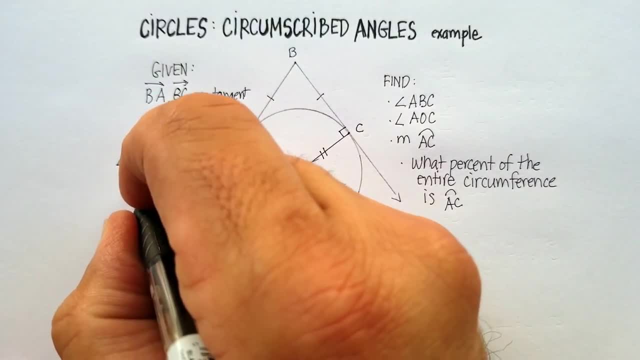 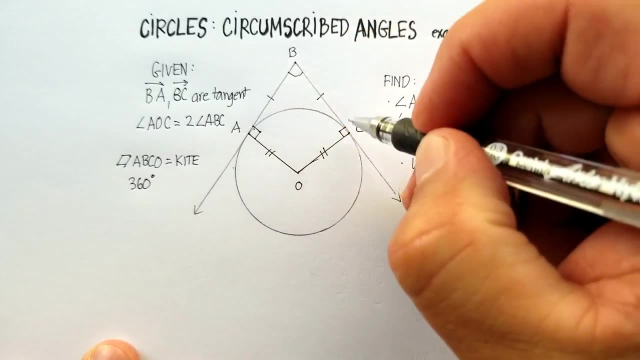 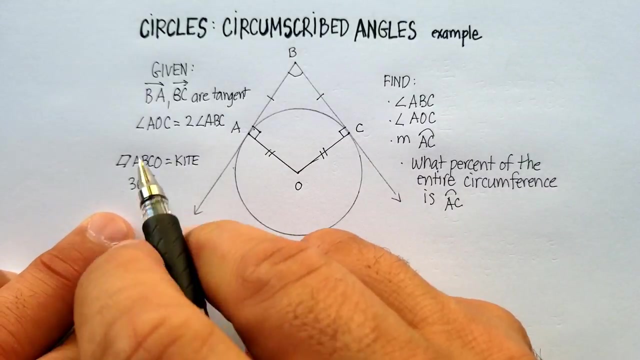 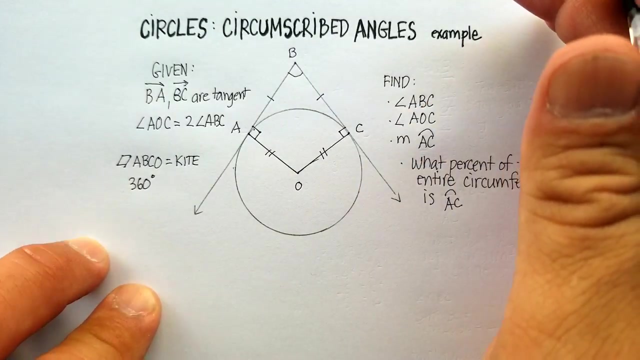 has 360 degrees internally. So if we were to measure this angle, this angle, this angle and this angle, it should add up to 360.. We also happen to know that this angle is twice as large as that one. Okay, so let's start doing some information here. We know. 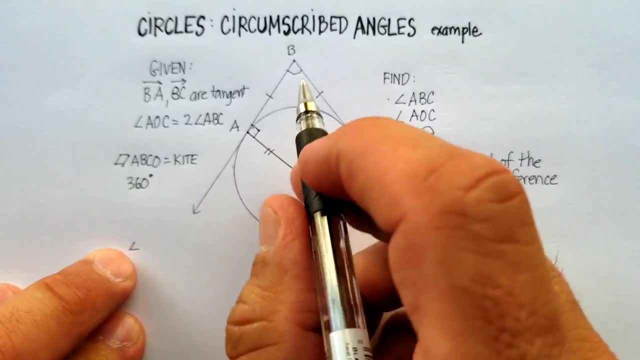 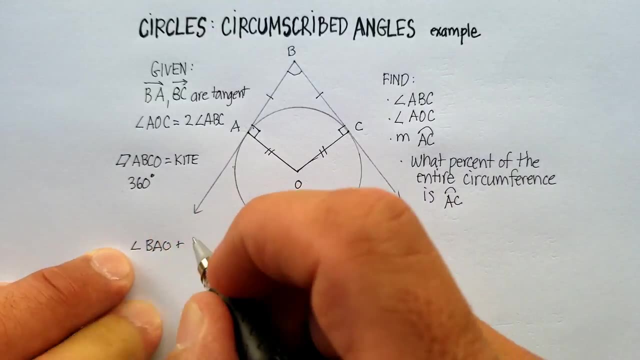 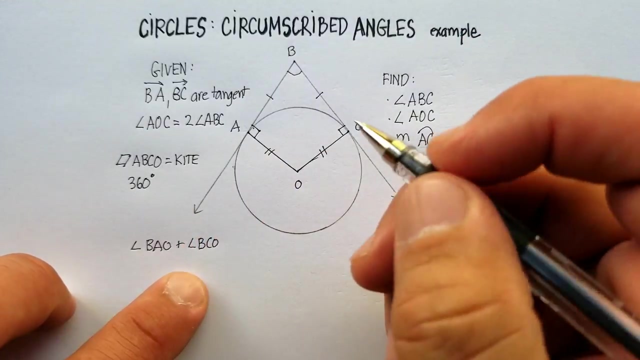 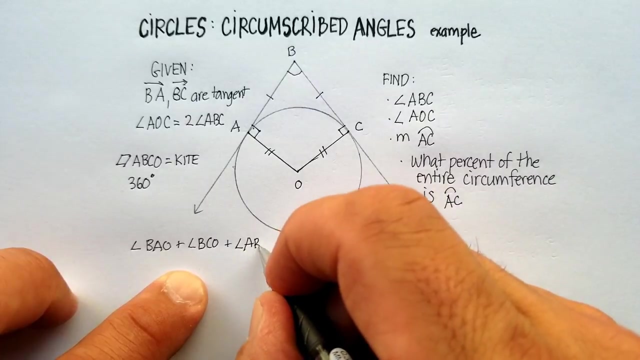 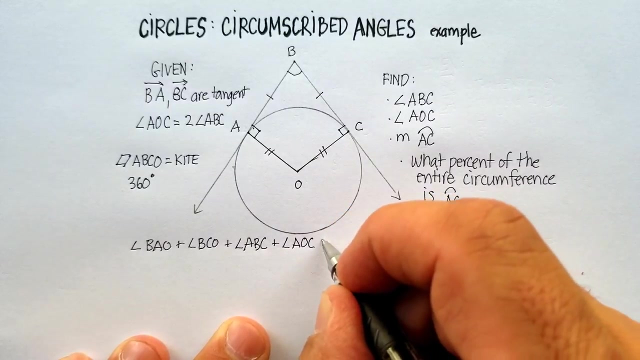 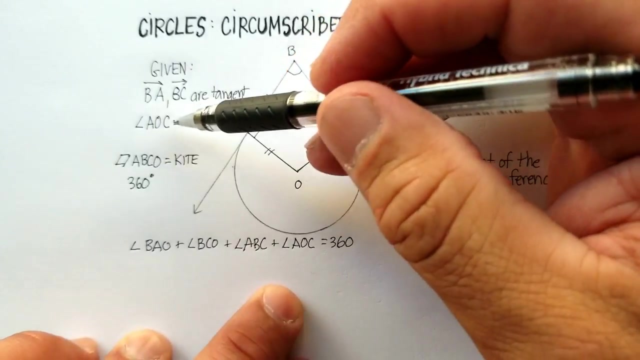 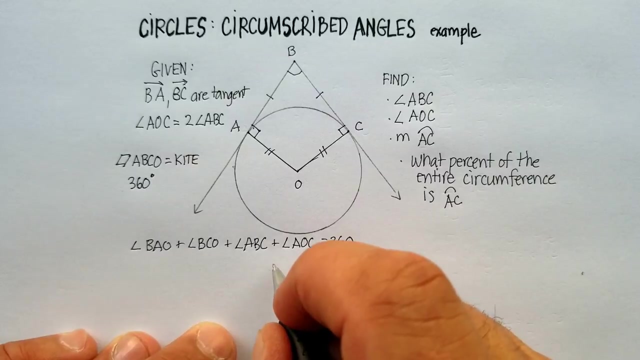 that Angle BAO plus angle BCO plus angle ABC plus angle AOC equals 360 degrees, don't we? We also know that we can replace angle AOC with two ABCs, So let's go down here and replace this with two ABCs. 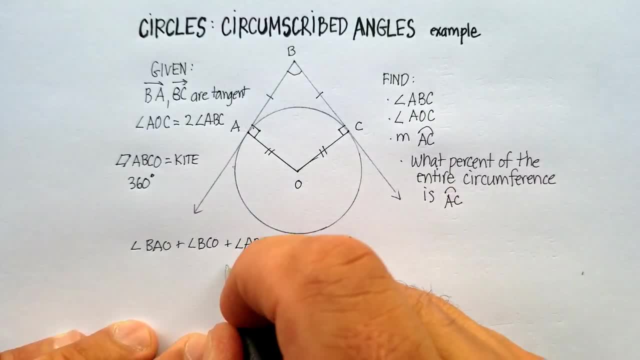 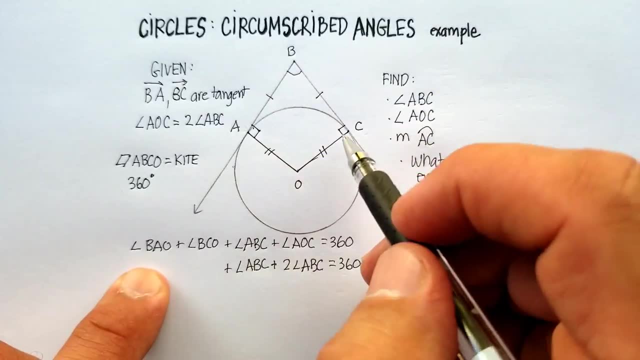 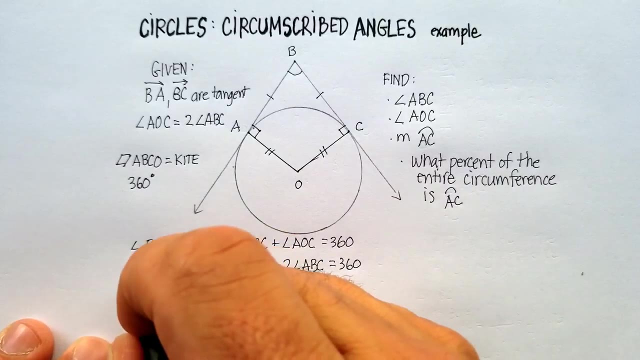 There we go, And we know that this is also there. We also know that these two angles are both 90 degrees, So let's put those in there as well. There's my first step. There's my second. Now let's keep on gathering our like terms. 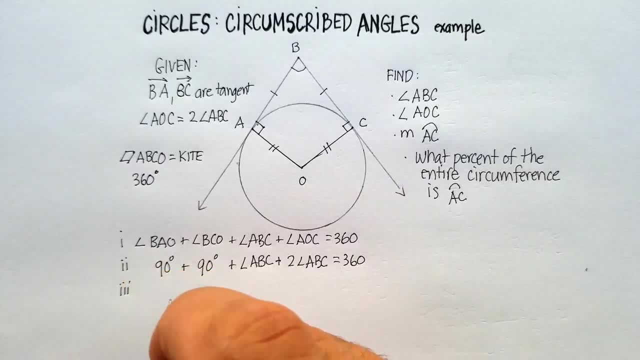 We know that 180 and 180, or, excuse me, 90 and 90 rather- is 180.. We know that we have basically three angle ABCs, And then we know that it equals 360 degrees. Let's subtract 180 from both sides. 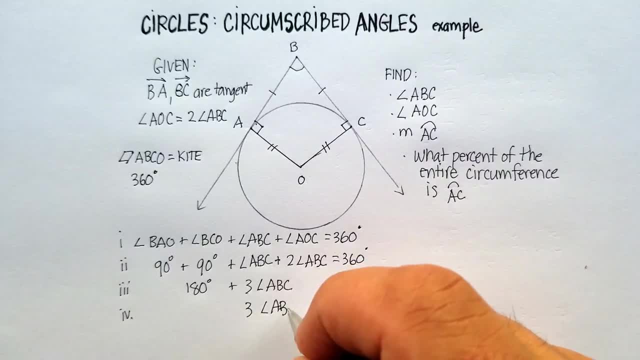 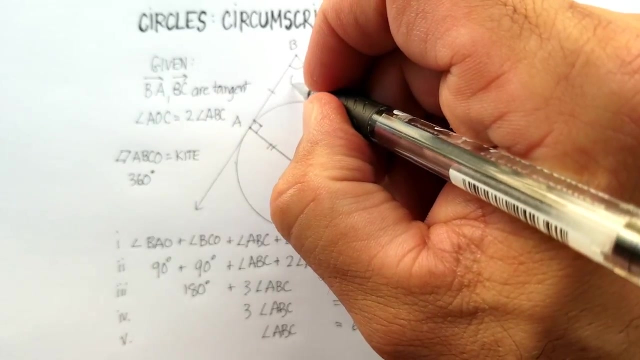 And we get three. angle ABC is equal to 180 degrees. And now let's divide both sides by three And you get angle ABC. Angle ABC is equal to 60 degrees. So let's go ahead and put that in there: Angle ABC is 60 degrees. 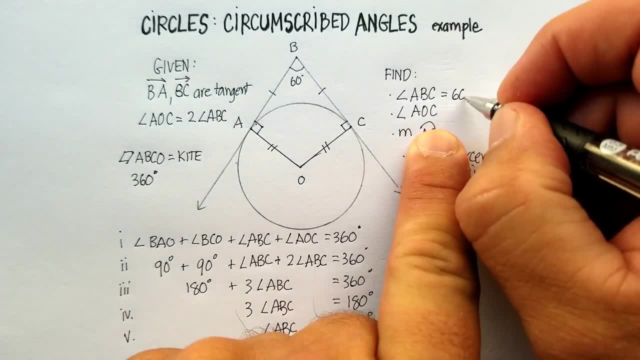 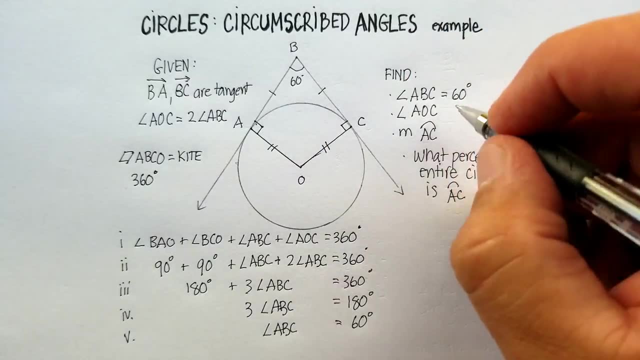 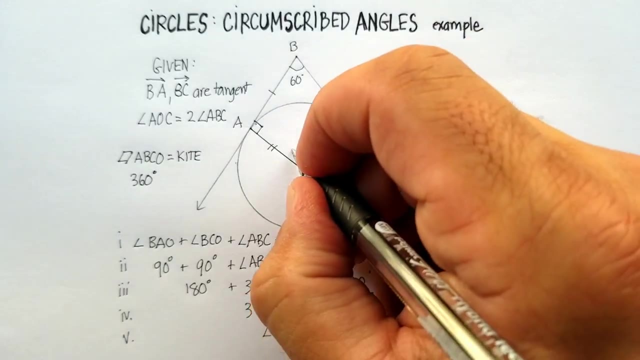 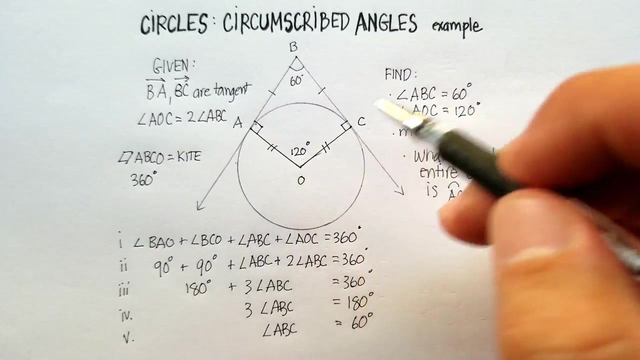 So we can actually put that as one of our first things that we have found. Now, if angle ABC is 60, angle AOC is two times that, which makes it 120 degrees. Now why is that important? Well, we know that angle AOC is a central angle, right? 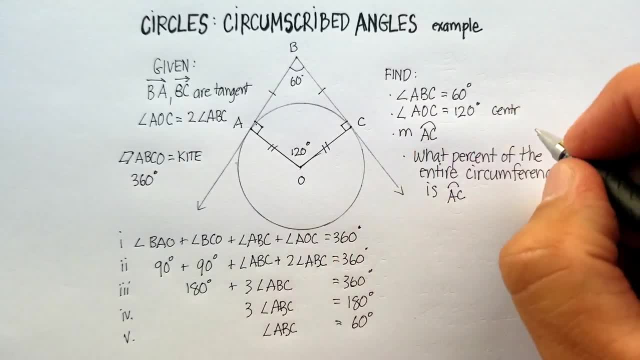 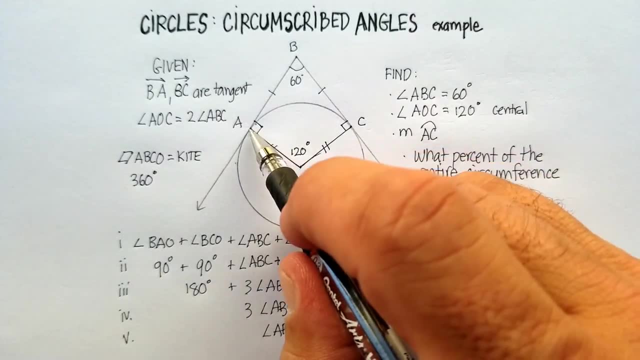 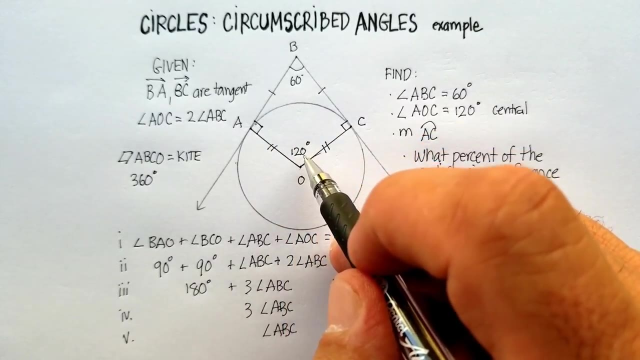 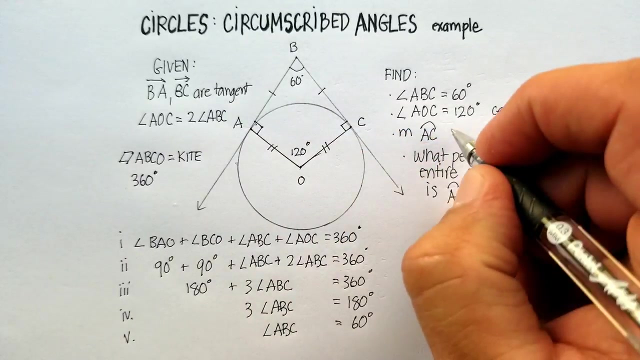 Because the vertex is starting in the center of the circle And the center of the circle, as it goes out, makes arc AC equal. to remember, that's called a central angle. That means that this Angle is the same as the number of degrees in that arc. 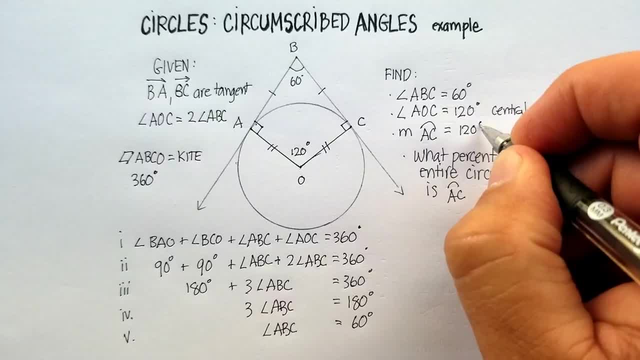 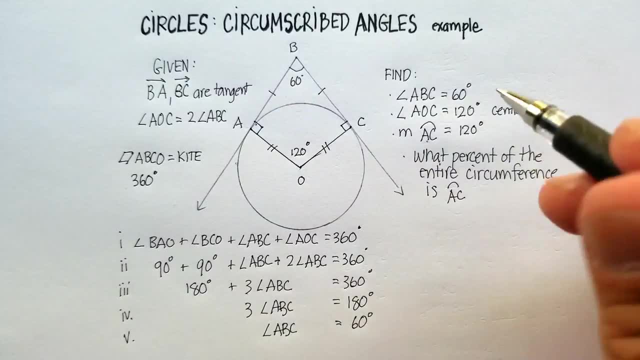 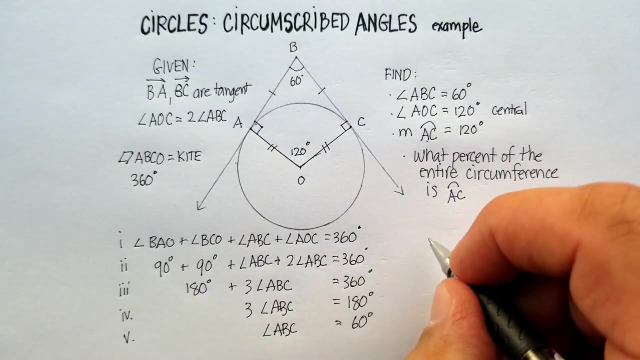 That's important. So it's 120 degrees For the measure of arc AC. So we've got that. Now we can answer the very final question: What percent of the entire circumference is arc AC? Well, we know the entire circle. 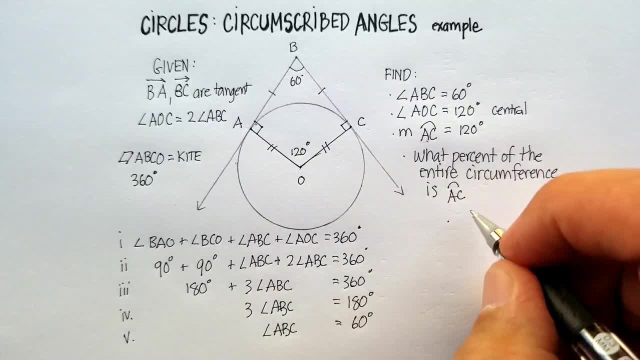 Let's go over here, Answer the question. We know that the entire circle is 360 degrees And the center of the circle is 360 degrees And the center of the circle is 360 degrees. We know that this portion is 120 degrees. 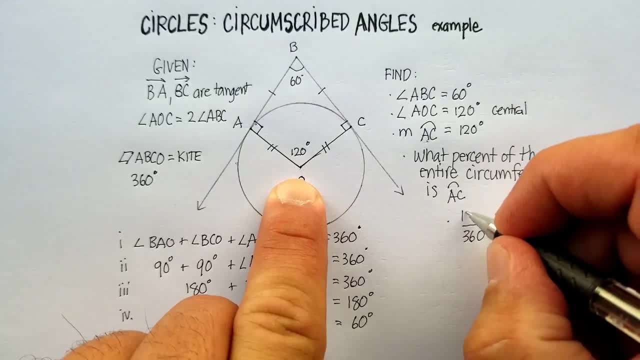 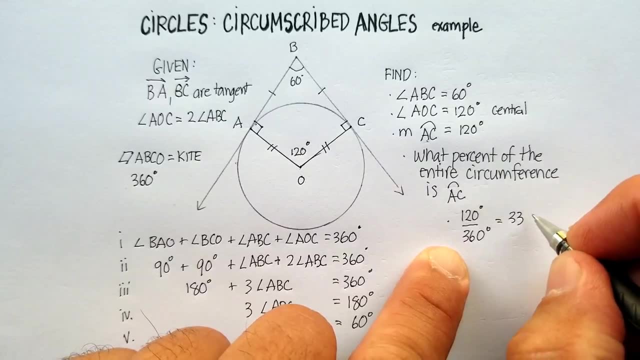 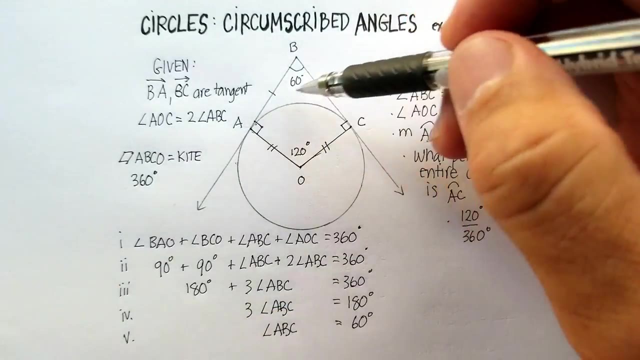 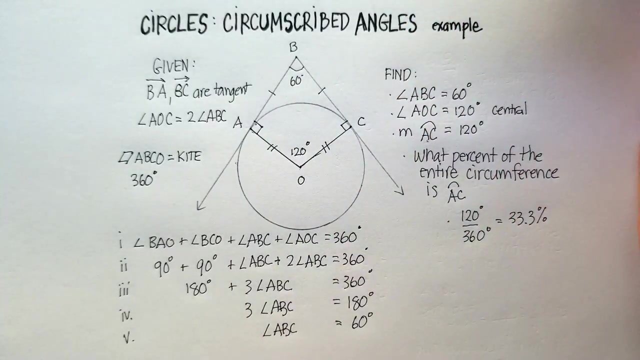 So therefore, 33 and a third percent is the answer to this arc. is that 33 or just a third of the entire circumference of the circle? Okay, I hope that was helpful.